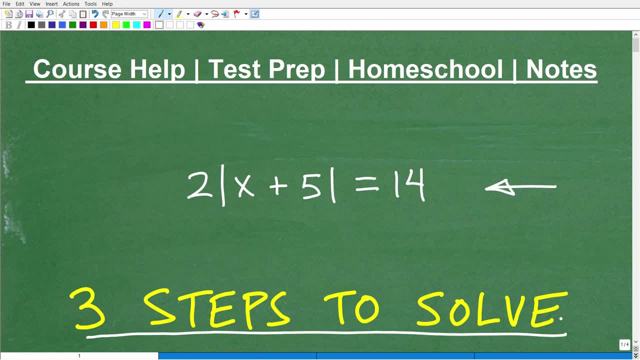 comment section. Of course I'm going to go through this and you can kind of check out and see how well you understand absolute value equations. And this isn't to be confused with absolute value inequalities. Oftentimes, when students are studying absolute value, 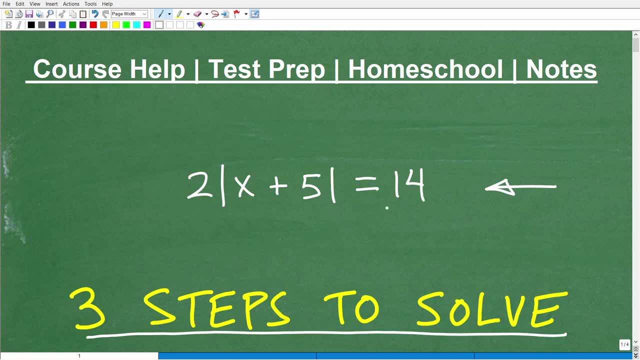 they learn how to solve absolute value equations and then they learn how to solve absolute value inequalities, and then they confuse the procedures, And so that's a pretty common mistake. So make sure, if you know what you're doing with this problem, that you're not using. 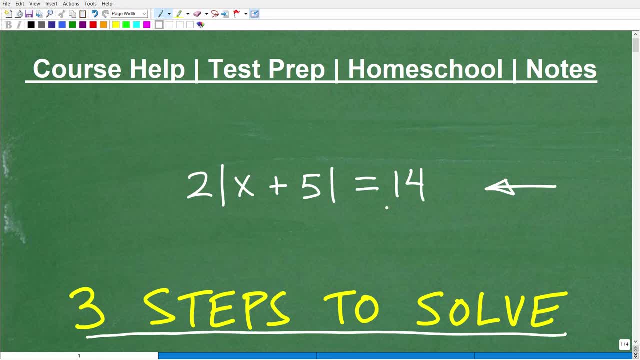 the procedures or the steps that we use in absolute value inequalities, And I'll do different videos on that, but we're going to focus in here on equations. Now I'm also going to review very quickly the basic concepts behind absolute value and absolute value equations. 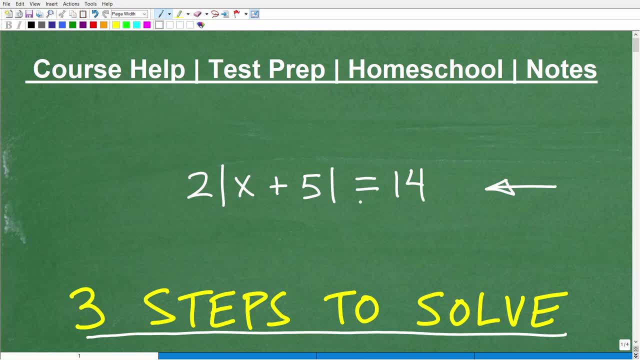 So we're going to get to all of this in just one second, But first let me quickly introduce myself. My name is John. I'm the founder of Tablet Class Math. I'm also a middle and high school math teacher. I'm going to leave a link to my math help program in the description. 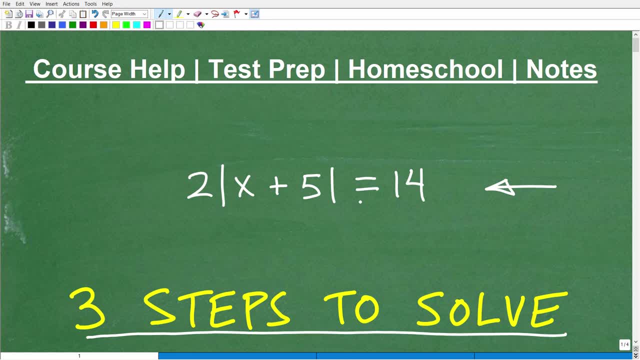 of this video. But if you're one of those students out there that is frustrated with math, maybe you don't feel like you're getting enough math instruction or enough practice where you really kind of understand what's going on, or maybe you don't really connect. 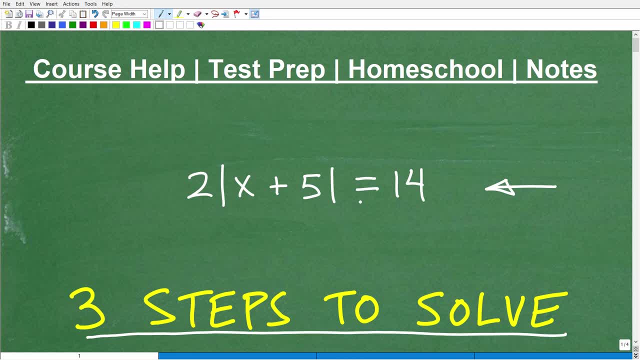 with your teacher's teaching style. Whatever the case might be, I've been teaching math for decades. I really pride myself on breaking things down in bite-sized, clear and understandable components. So if you're at the middle school, high school or even college level in terms 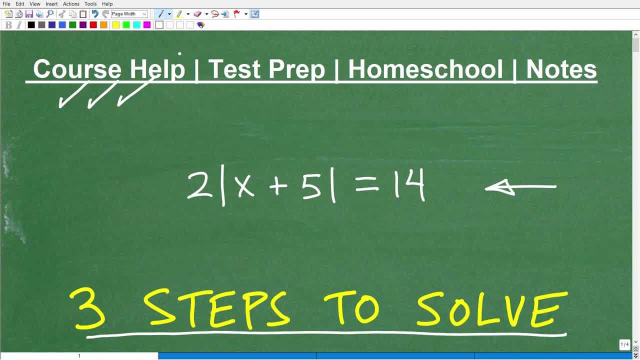 of mathematics. I can help you succeed in your respective math courses. Now, if you're taking any test or you're scheduled to take a test that has a math section on it- I'm talking about things like the GED, SAT, ACT- 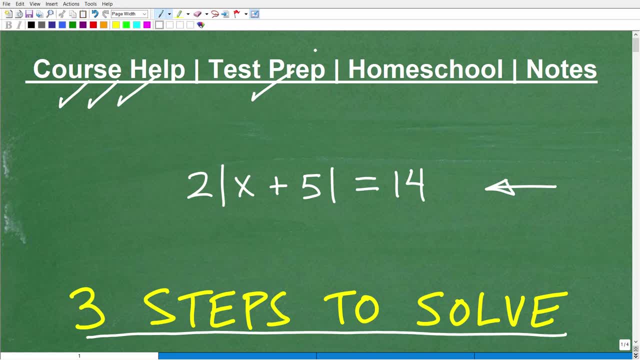 GRE, GMAT, ASVAB, ACCUPLACE or ATLEX exam, Maybe a teacher certification exam, You get the idea I can help you prepare and pass those exams. If you homeschool definitely got to check out my whole entire homeschool math program- Very, very comprehensive, I've. 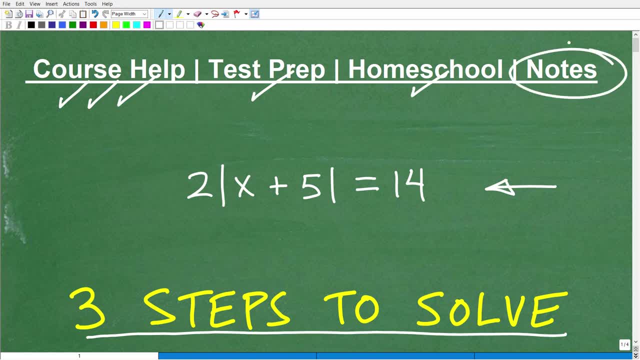 been working with homeschoolers for many, many years. And if you don't have any math notes, don't panic, I'm going to leave the links to my math notes in the description of this video. But if you want excellent grades in math, if you want like those top fantastic. 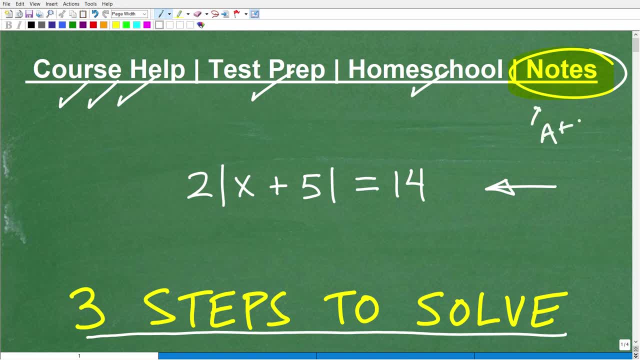 A pluses and whatnot. You have to take great math notes. So there's just no way you're going to be successful in math without taking excellent math notes. Okay, so let's get to our problem here Again, if you think you know how to do this problem, 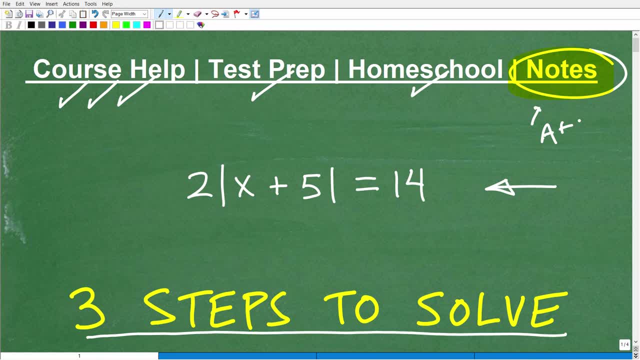 go ahead and pause the video and just don't look at your notes, Don't just? this should be something that you have in your memory. Now, if you take in any um or if you are taking an algebra course, you're going to have to know how to do this, And and again. 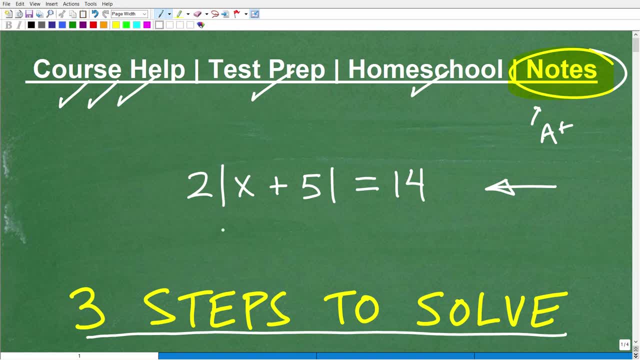 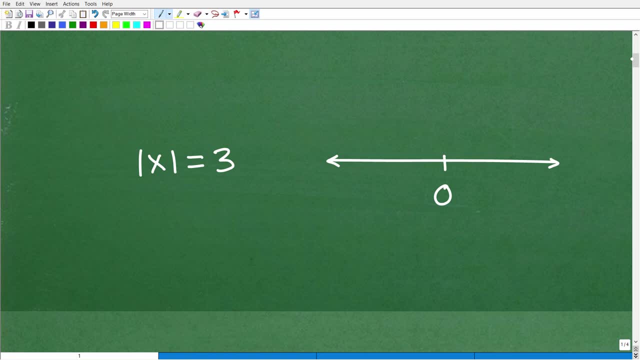 if you've taken algebra, you already learned this, and this is going to come up over and over again. So I'm going to go ahead and review a basic problem with you. Then we'll get into the actual problem here. So let's take a very simple problem. The absolute value of X is: 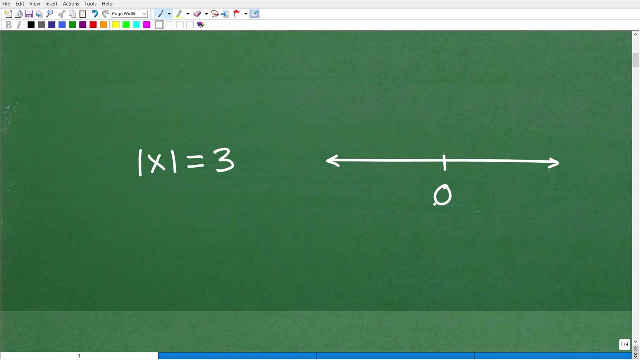 equal to three. Well, you can see, here I have a number line and this is zero. So what is the absolute value? So, in other words, if I went absolute value of three, okay, what does that equal to? Well, hopefully most of you out there be like, Oh, that would be equal. 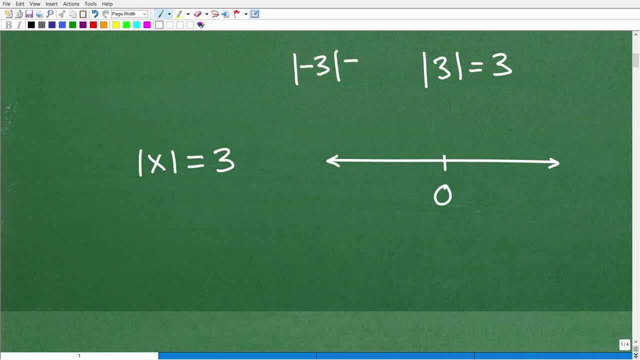 to three. Now, how about the absolute value of negative three? What does that equal to? Well, hopefully all of you are like: isn't that equal to three as well? You would be correct. So negative three and three. okay, On the number line, the absolute value tells us. 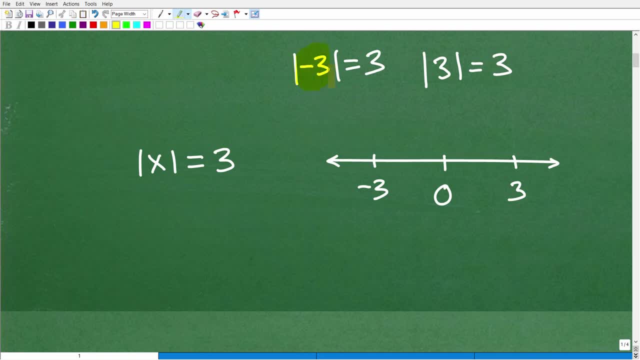 the distance a number is from zero. So right here, when we're taking absolute value of negative three, we're really asking a question: How far is negative three from zero on a number line? Well, it's three units away. How far is three from zero on the number line? Well, it's also. 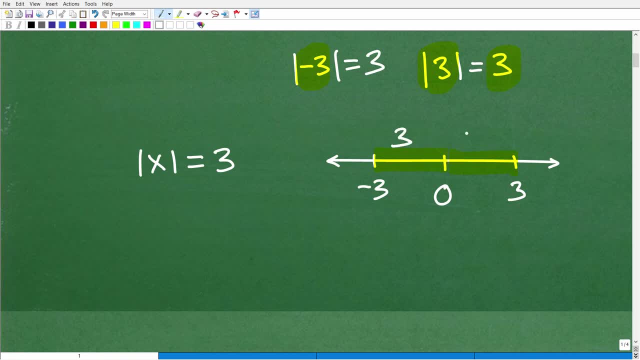 three units away. So that's what absolute values is. The absolute value of three is equal to three, and three is from zero on the number line. Well, it's three units away. Well, it's absolute value represents, again, it's the distance a number is from zero on a number line. that's why 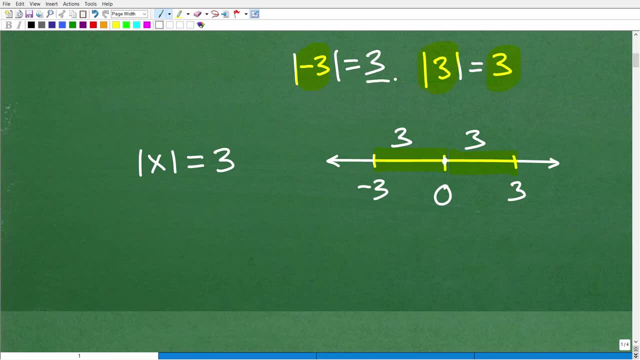 the absolute value of a negative number is positive because, remember, we measure distance in positive units. okay, so now, knowing that we can take a look at this equation, okay, the absolute value of what number is equal to three? well, we just kind of saw here that if we take the absolute 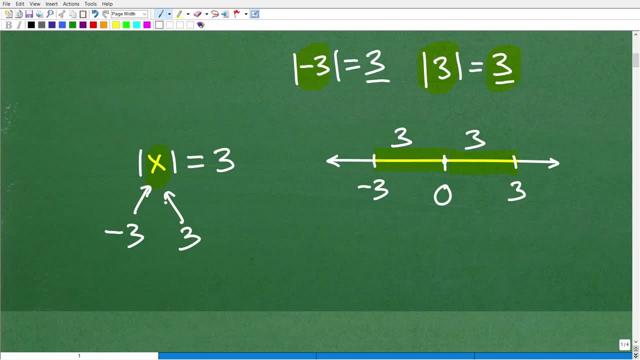 value of negative three and the absolute value of positive three. okay, both of these numbers here will give us the answer of three. so when you're solving absolute value equations, remember that you're always going to have two answers. so in this case, x is equal to negative three and x is also. 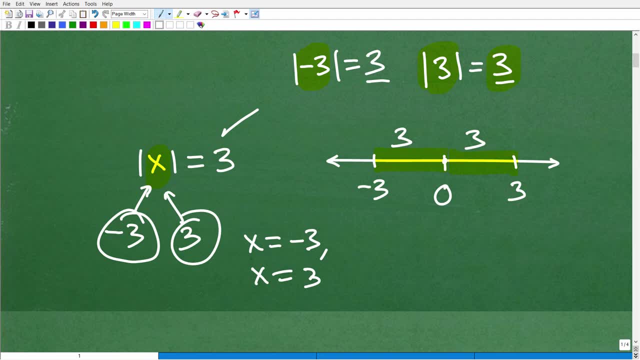 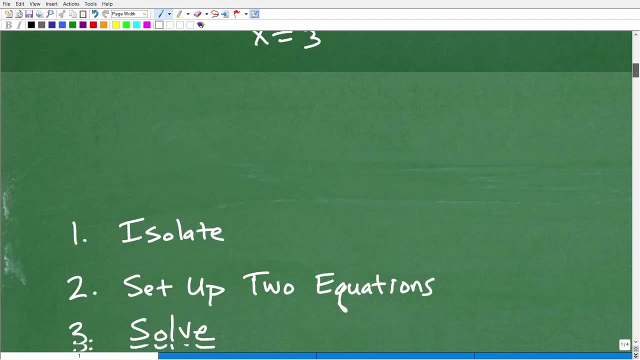 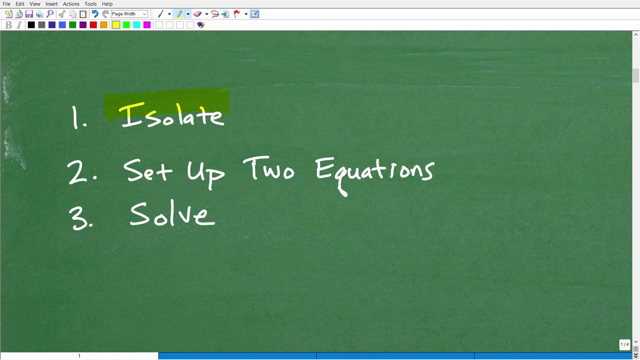 equal to positive three. okay, so just a quick basic review of why we're going to do what we're going to do next, and i'm going to show you the steps to solve um absolute value equations. and the first step- oops, i didn't do that, uh- is to isolate. we need to 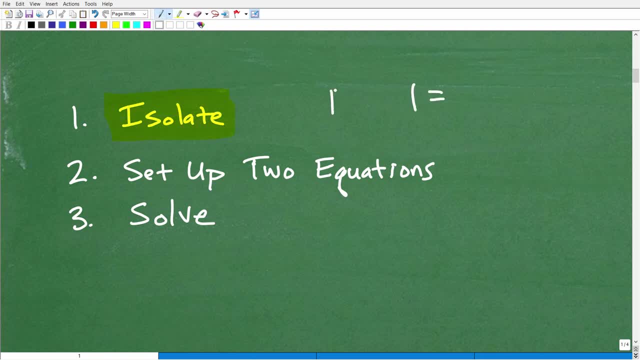 isolate the absolute value part of the equation and we want one number on the other side. now this might require a couple, two or three different kind of subsets, but the main step here is to isolate the absolute value equation part and we want to have one number on the other side of that. 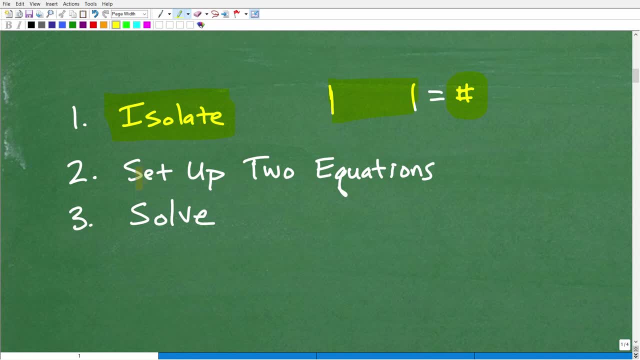 i'll show you exactly what i'm talking about here in a second. now the second step is we're going to set up two respective equations, and then the last step here is we're going to solve. so these are the three main components to solving an absolute value equation. so let's get into the 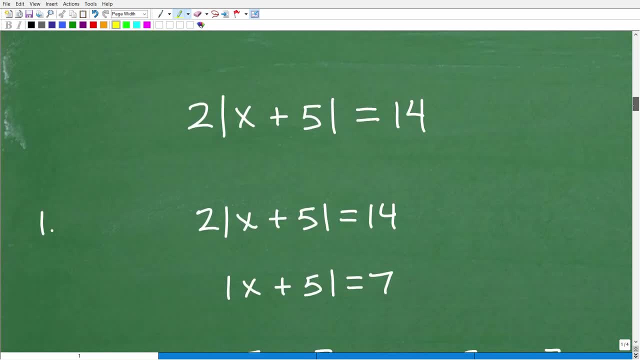 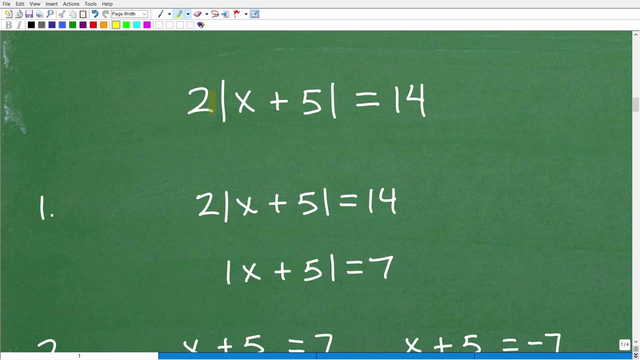 actual problem here and we'll see what i'm talking about. okay, so here is the problem: two times the absolute value of x plus five is equal to 14. now, one of the things that a lot of students do- uh, it's a very common mistake- is they? they think they have to do the distributive property, or? 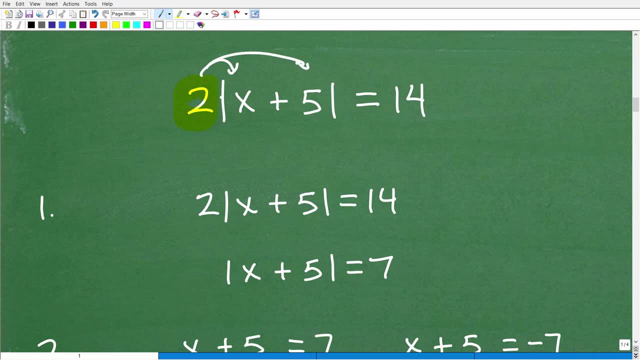 they think they can. they confuse this absolute value function with, like a grouping symbol, like two times x plus five is equal to 14, and then they go: oh, 2x plus 10, they. they try to solve this like an equation, an actual equation. that's not the case. remember, you cannot distribute this outside. 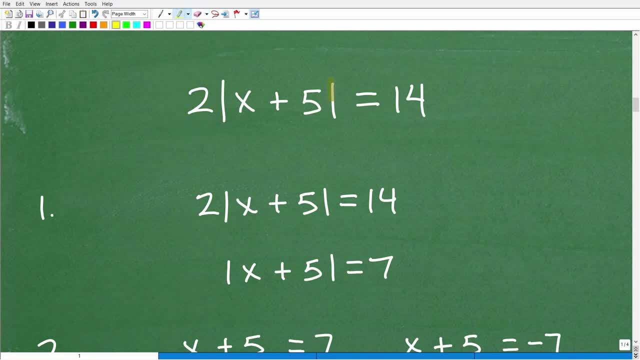 number here, but our main goal is to isolate. we want to isolate this absolute value part of the problem. so how can i do that? i have two times the absolute value function and i'm going to divide both sides of the equation by two. okay, when i do that, i'm going to get. seven is equal to the. 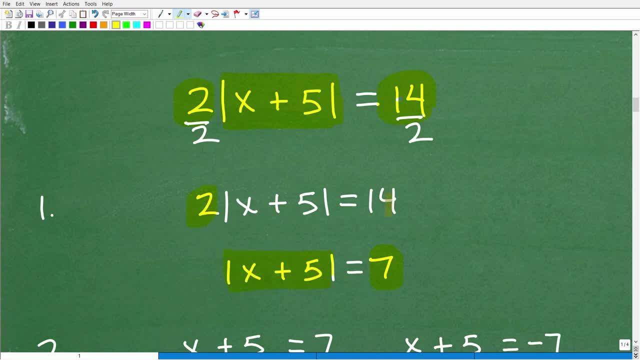 absolute value of x plus five. okay, so i'm just dividing both sides of this absolute value function by two and i get seven is equal to the absolute value of x plus five. so this is the first uh part, or the first step is to isolate this absolute value function on the left hand side. 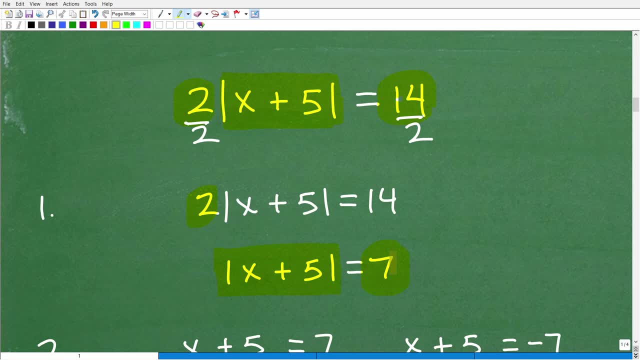 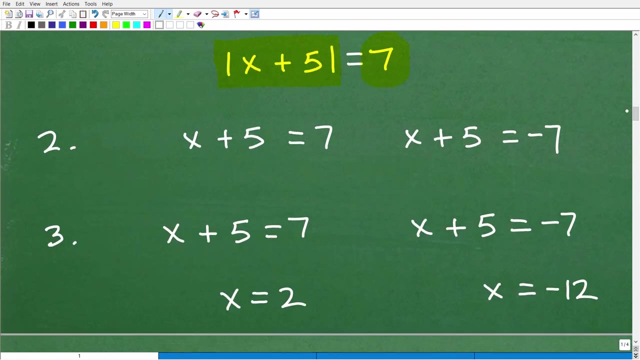 and then we're going to have one number on the right hand side. now, sometimes you have to do a few more additional steps in this isolate- uh- part of the problem solving process, but this is what we are talking about. so, once we're done isolating, we're going to move on to step two, and step two is to 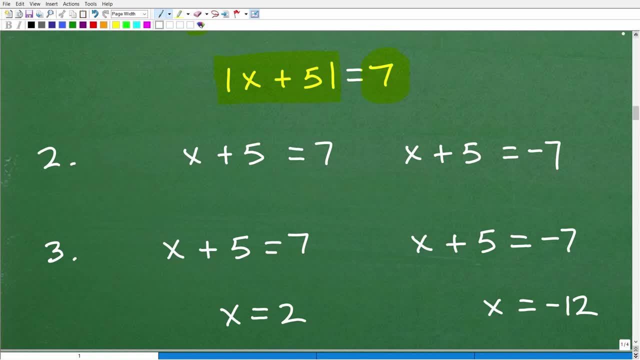 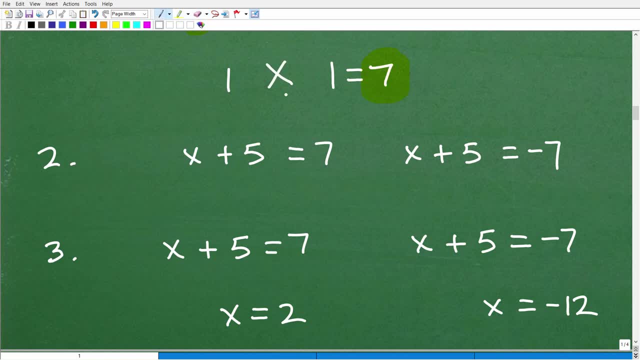 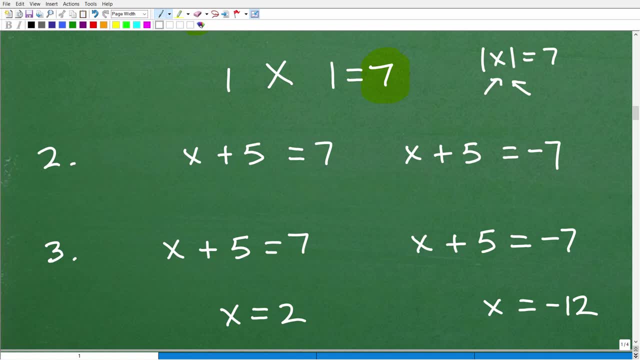 already saw an example, this um can x be? in order to get an answer of absolute value of some number is equal to seven. what can these? what can x be? well, hopefully you say, oh, x could be seven or negative seven, and we would be correct, okay, so 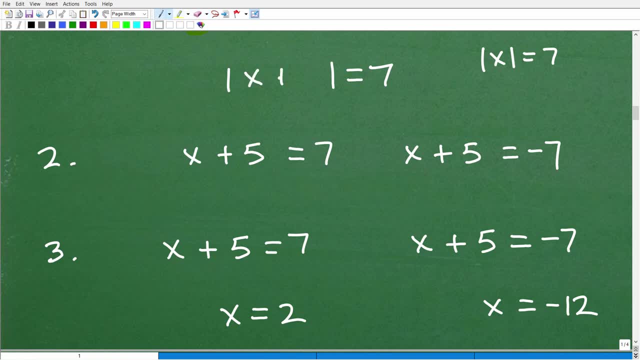 let's go back to our problem. absolute value of x plus five is equal to seven. all i know is this: x plus five. i know what you are. you're either a seven or a negative seven. okay, that's the only way we can get an answer of this. absolute value of some expression here is equal to seven, so you. 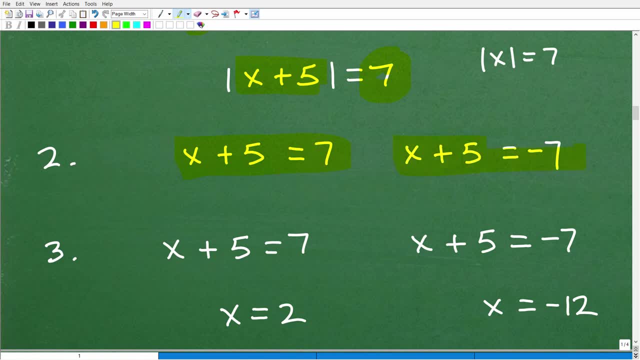 say: okay, x plus five, you're either seven, or x plus five, you're either negative seven. so this is our second step. we're going to set up two equations and we're going to set up two equations, okay. so we're always going to get two answers when we're solving absolute value equations. so 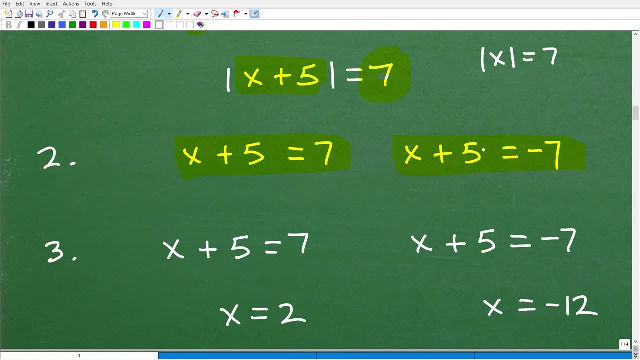 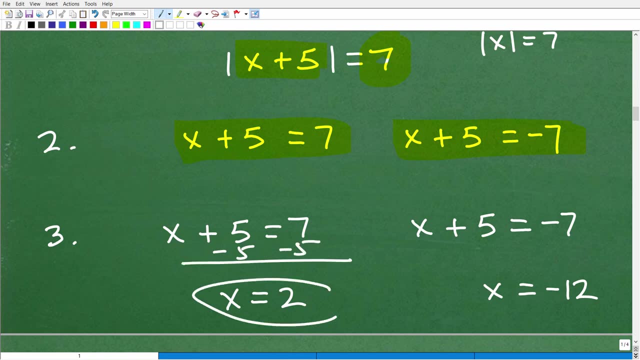 this is our setup for our two respective equations, and then we're going to go ahead and solve those equations. here we have: x plus five is equal to seven. i simply subtract five from both sides of the equation. i get x is equal to two, and here i'm going to subtract five from both sides of the.